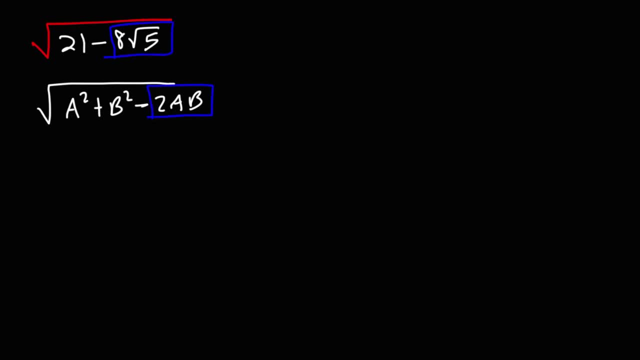 8. square root 5 has to equal 2ab. So if b is equal to the square root of 5, that means that 8 has to equal 2a. So if 2a is equal to 8, divide them both by 2, that means a. 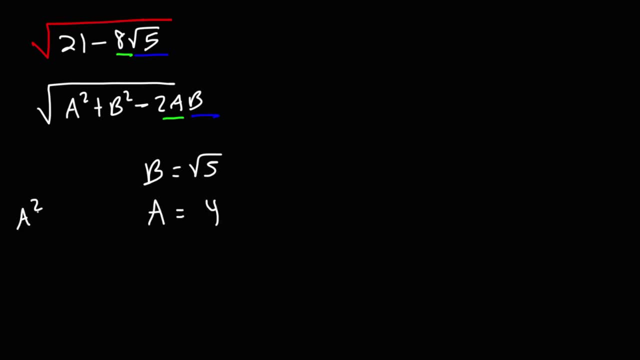 is equal to 4.. If a is 4, a squared is 16.. And then that means b squared. If you square the square root of 5, you're just going to get 5.. Notice that a squared plus b squared adds up to 21.. 5 plus 16 adds up to 21.. 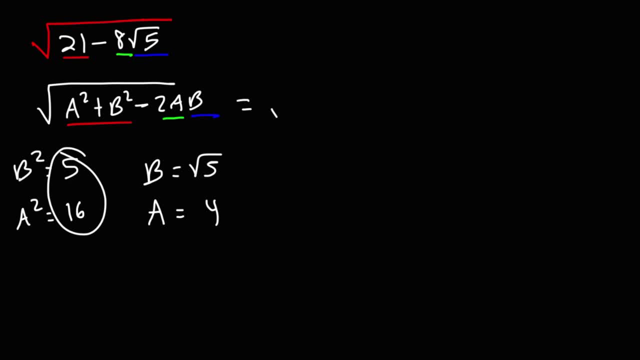 Now we know that a squared plus b squared minus 2ab, that's going to be a minus b squared, which all of this simplifies to a minus b. So we know that a is 4, b is the square root of 5.. 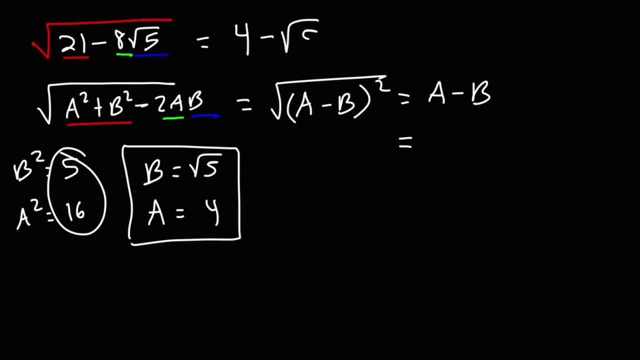 So it's going to be 4 minus the square root of 5.. This, right here, is the answer, And here's how we can check it: 4 minus the square root of 5 squared should equal what's inside of the radical 21 minus. 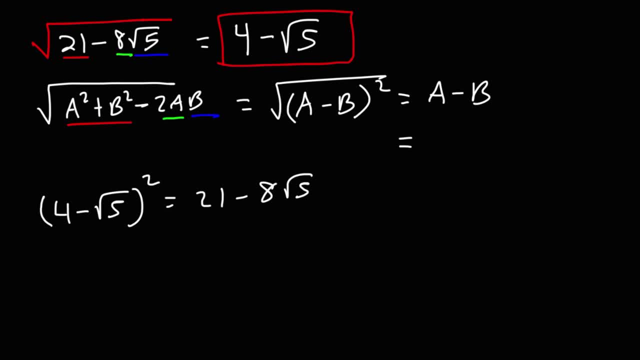 8, square root 5.. Because if you take the square root of both sides then you're going to get a square root of 5 squared. So if you square the square root of 5 squared, then 4 minus the square root of 5 should equal our original expression. 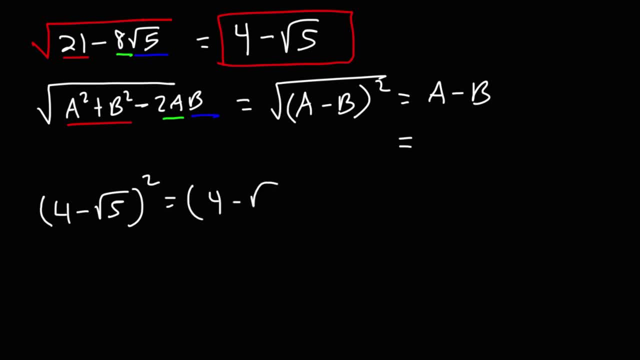 So what we're going to do is we're going to FOIL this expression, We're going to multiply 4 minus the square root of 5 by itself. So 4 times 4, that's 16.. And then here we get negative 4, square root 5, and another negative 4, square root 5.. 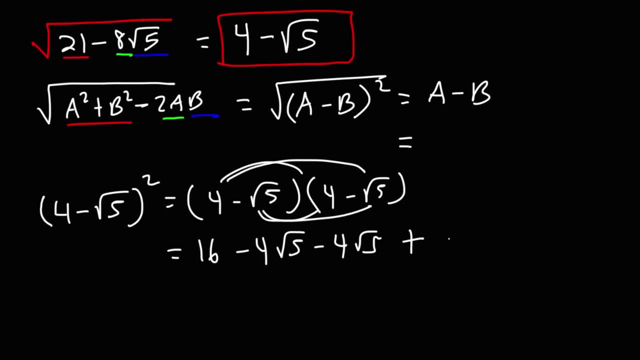 And then 2 negatives, We'll make that 4 minus the square root of 5 squared. If we make it positive, the square root of 5 times the square root of 5 is the square root of 25, which is 5.. 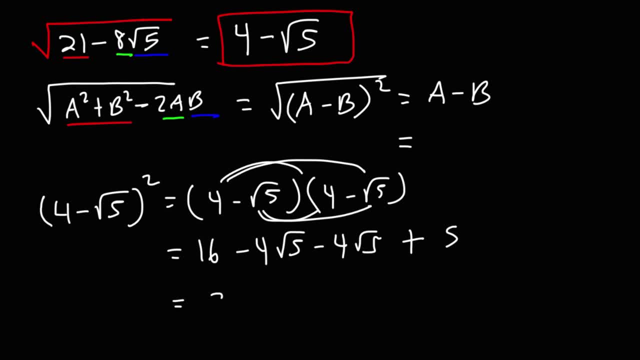 So, combining the first and last terms, we're going to get 16 plus 5, which is 21.. And then negative 4 minus 4,, that's going to be negative 8.. So we do get what's inside of the radical, which means this is indeed the correct answer. 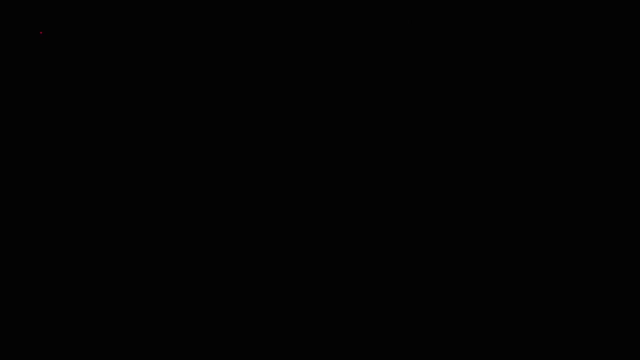 Now, for the sake of practice, let's try another one. Go ahead and try this one. Let's say we have the square root of 5, squared Square root of 16 minus 6, square root 7.. So go ahead and use the process that we've used earlier to simplify this radical expression. 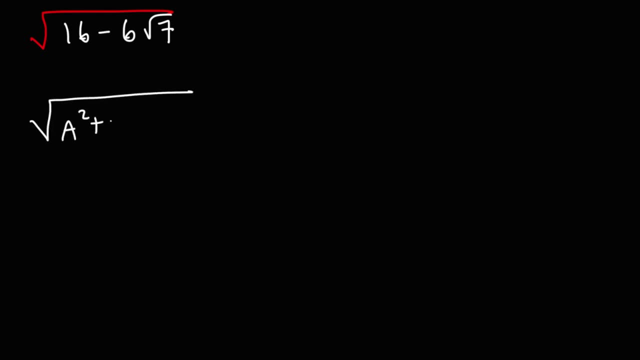 So we're going to see if it's in a form a squared plus b squared minus 2ab b. So let's assume that b is equal to the square root of 7.. If that's the case, 6 has to equal 2a. 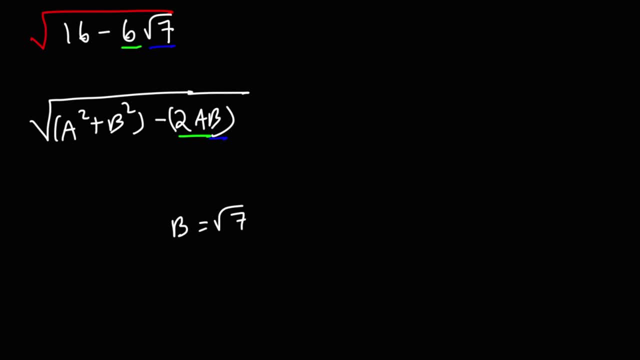 If 6 is equal to 2a, 6 divided by 2 gives us a, which is 3.. And so that means a squared is going to be 3 squared, which is 9.. b squared is going to be the square of the square root of 7, which is 7.. 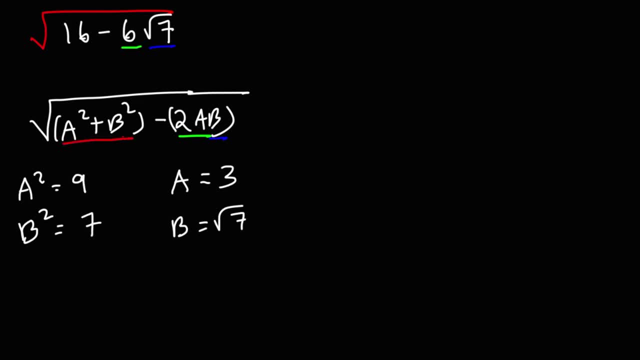 And now we need to make sure that a squared plus b squared is equal to 6ab, Which it is because we can see that 9 plus 7 is 16.. So that tells us that we could use this formula. We have it in the form: a squared plus b squared minus 2ab. 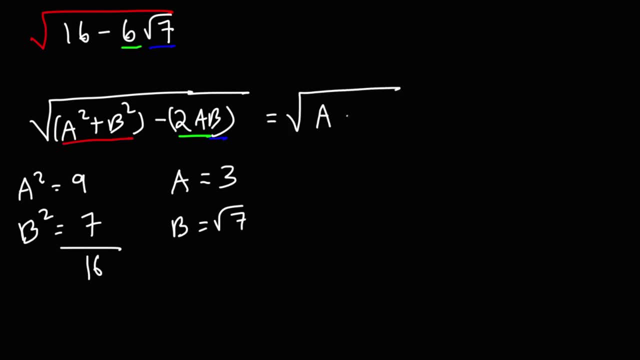 So this is going to be the square root of a minus b squared, which simplifies to a minus b. So our final answer is just going to be a minus b. a is equal to 3.. b is equal. b is equal to the square root of 7.. 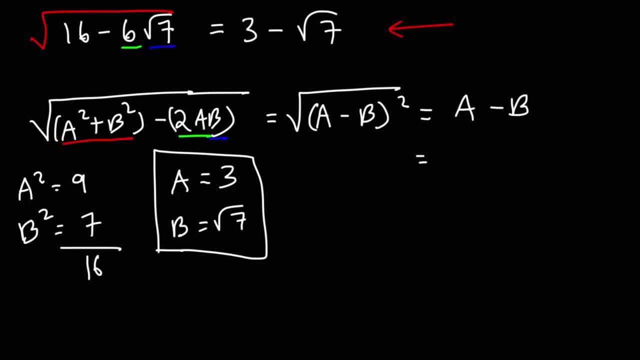 So all we need to do is simply check this answer Just to make sure we have the right answer. So let's FOIL 3 minus the square root of 7 times itself. So 3 times 3, that's going to be 9.. 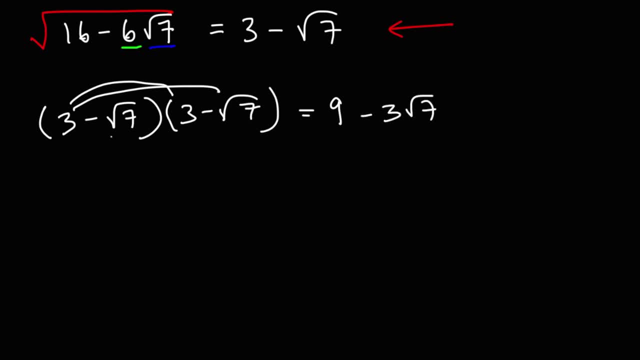 And then we have 3 times the square root of 7. And then multiplying those two will give us the same answer. And then finally, negative root 7 times negative root, 7 will simply be positive 7.. So, combining like terms, we have 9 plus 7, which is 16.. 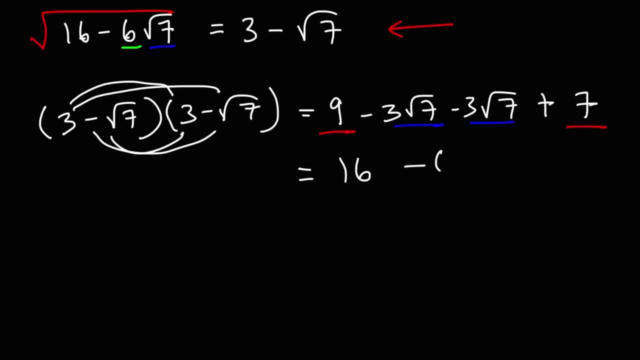 And then negative 3 minus 3, that's going to be negative 6, with the square root of 7 attached to it. So, as we can see, we get what is inside of the square root symbol, Which means this answer is indeed correct for this example problem. 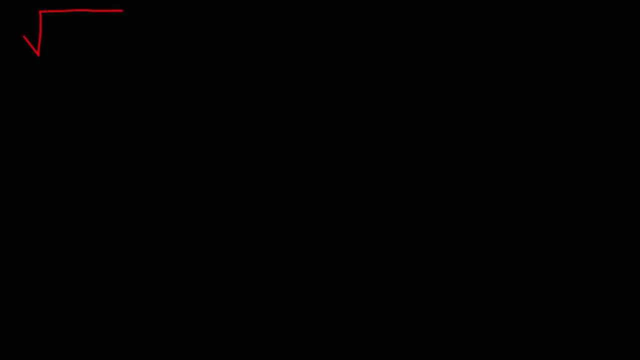 Now let's work on one final problem. So this is going to be the square root of 39 plus 12 times the square root of 3.. Go ahead and pause the video and work on this problem. So this time we have a plus symbol instead of a minus symbol. 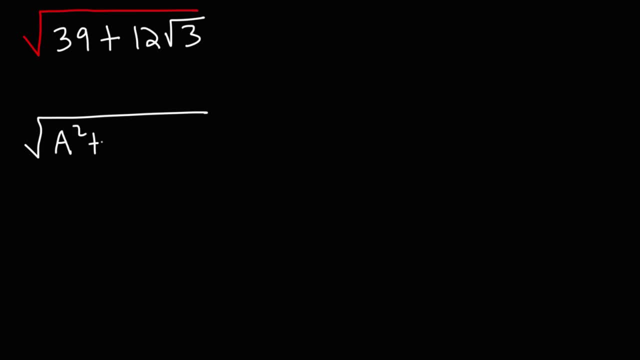 So we're going to use this formula: a squared plus b squared, but plus 2ab. So let's assume that b is equal to the square root of 3.. That means that 12 has to equal to 2a. So 12 divided by 2 will give us a, which is equal to 6.. 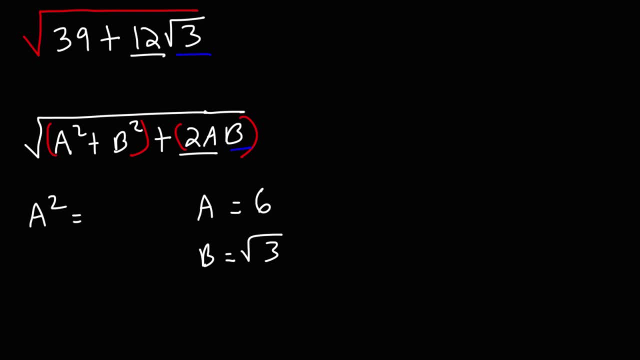 So, a squared, that's going to be 6 squared, which is 6 times 6.. That's equal to 36.. And b squared, the square root of 3 times the square root of 3,, that's the square root of 9, which is 3.. 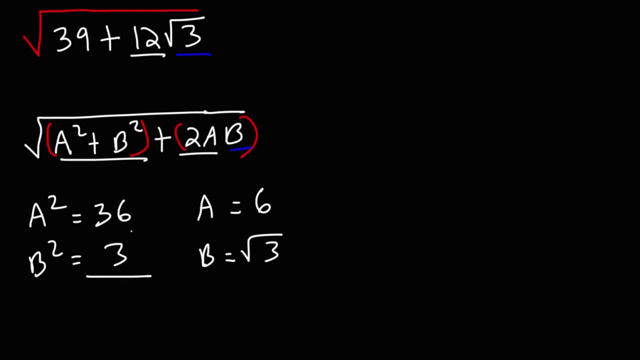 And so, a squared plus b squared, we could see that 36 plus 3 gives us 39. So these numbers fit this formula. So this is going to simplify to the square root of a plus b squared, which will give us the final answer: a plus b. 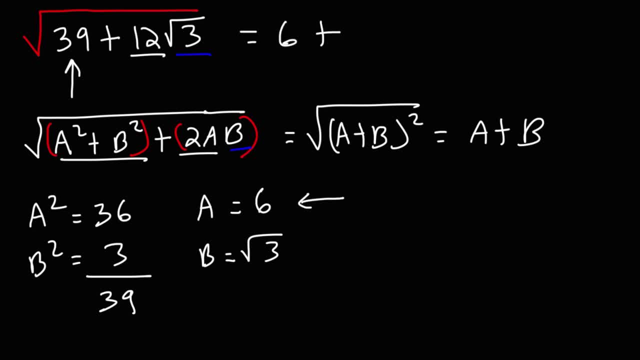 So a is 6, b is the square root of 3.. So our final answer should be 6 plus the square root of 3.. Now we know the answer is going to be correct, but let's go ahead and make sure.